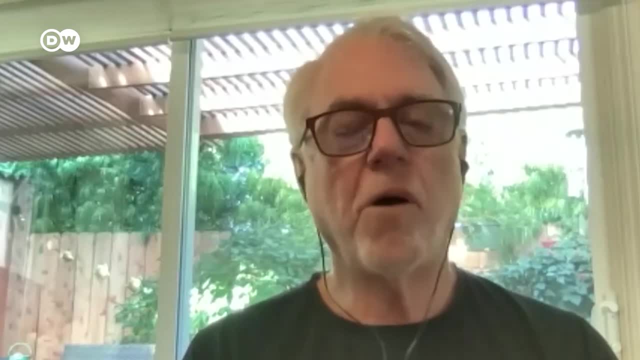 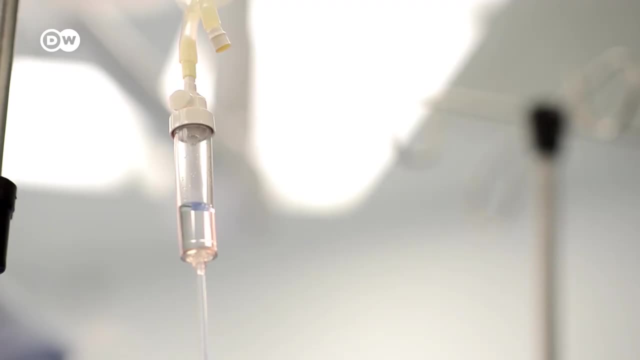 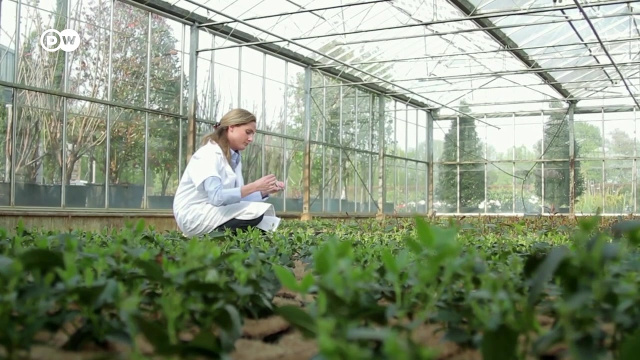 has been used to treat cancer. It's been elaborated on and altered to give it good properties as a medicine. Some 70% of cancer medications alone are based on nature, according to UN experts, But the search for new sources of pharmaceuticals is becoming ever more difficult. 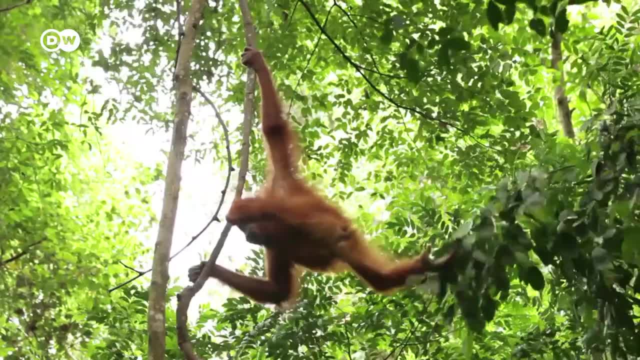 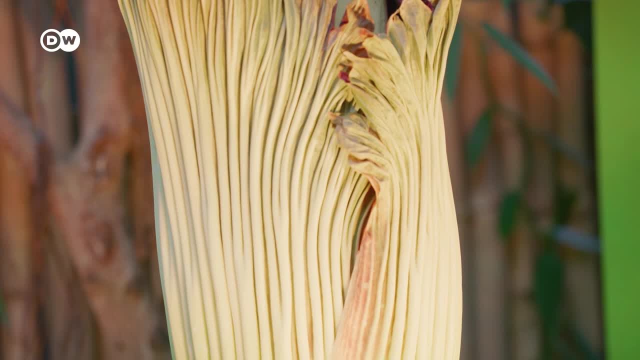 Biodiversity is disappearing at an alarming rate. Almost a third of more than 150,000 species assessed as part of the IUCN's red list, which tracks the state of the world. The world's biodiversity are threatened with extinction, And humans are to blame. 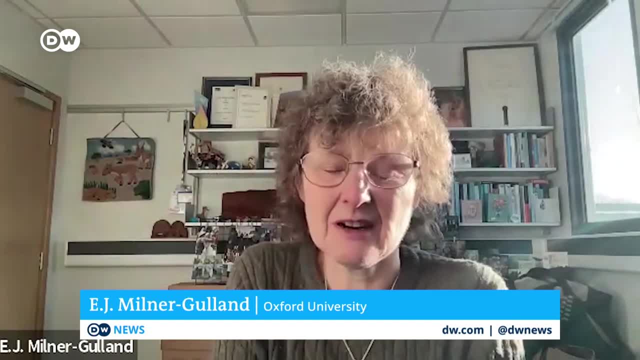 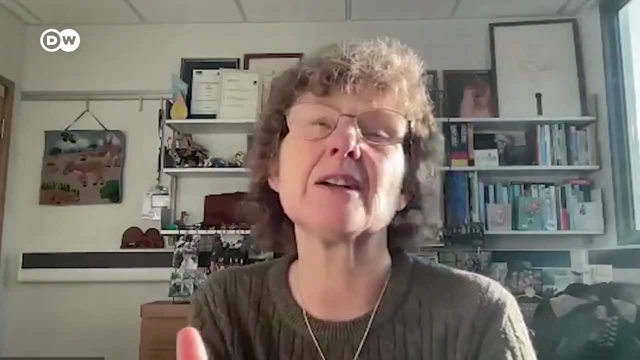 The two things that threaten biodiversity the most at the moment are over-harvesting and land conversion. And that's not just clearance of land for livestock to graze, it's clearance of land for food for livestock to eat and clearance of the oceans. 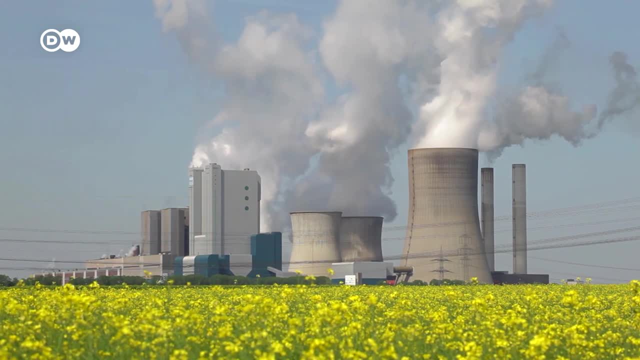 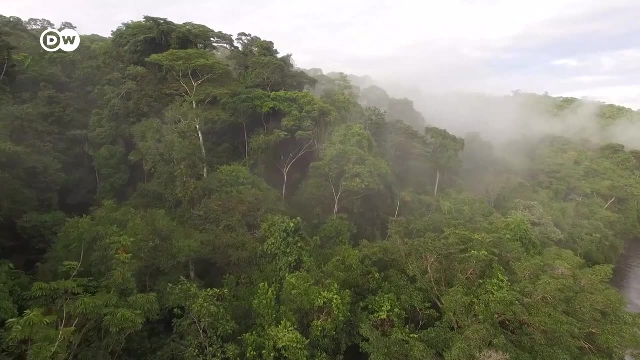 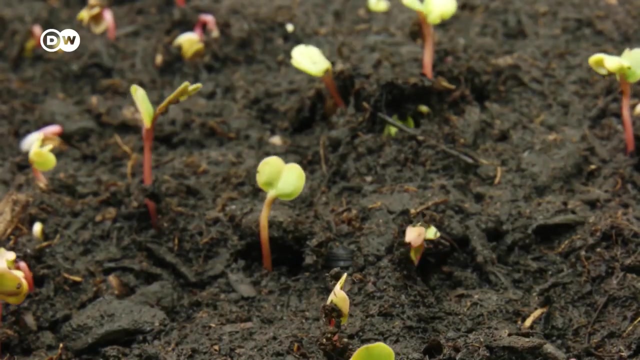 Human-driven climate change is also having an impact. Scientists say loss of biodiversity. it does not just present a problem for a drug discovery. Humans are almost completely dependent on the natural world, whether it's through trees that remove pollutants from the air or crops that provide food. 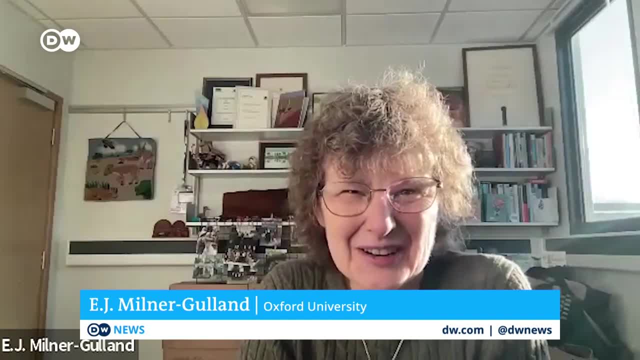 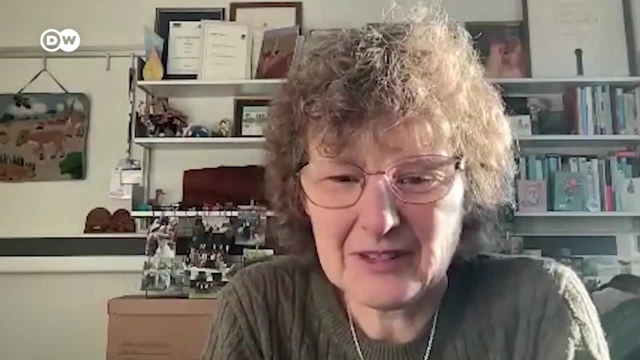 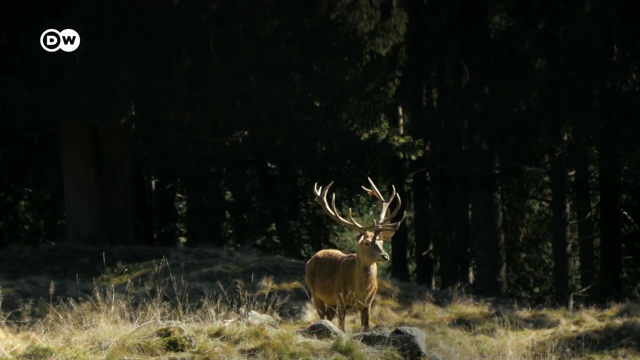 The biodiversity is the fabric that holds our life support together on our planet, And if we didn't have living wild nature, it would be much harder or impossible to live on this planet. Governments have promised to tackle biodiversity by protecting 30% of land and oceans before 2030.. 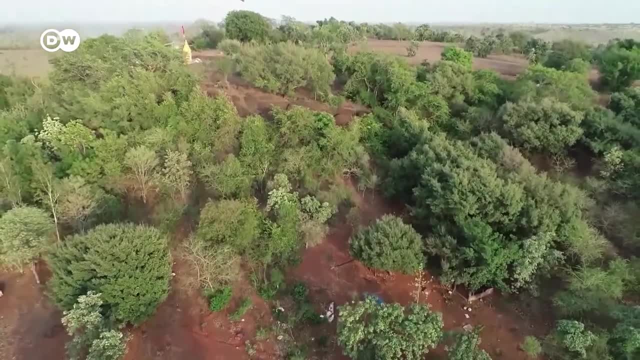 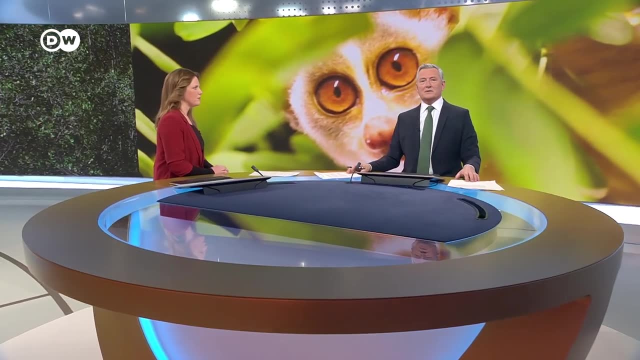 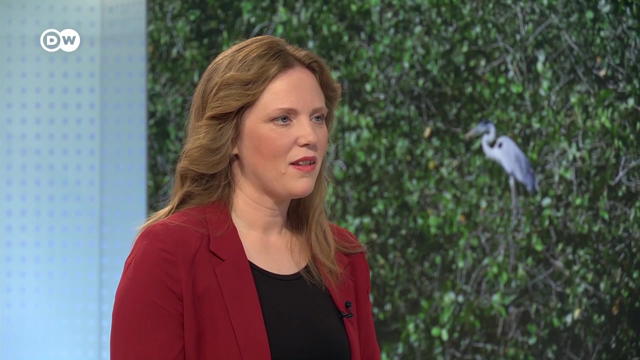 Whether the commitments become action could dictate not just the state of the planet but also human health, And with me in the studio is Louise Osborne from DW's Environment Desk. She filed that report. of course, Louise, we heard in your report about how biodiversity is extremely important for pharmaceuticals and also for food. 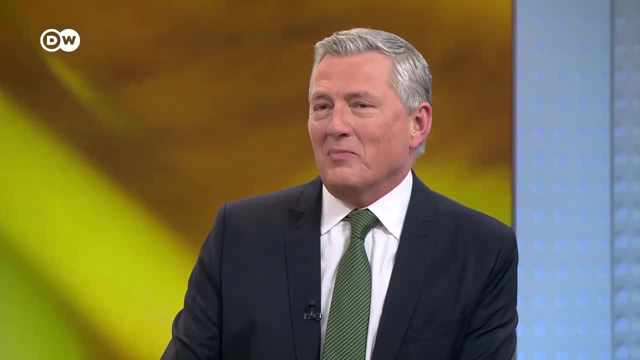 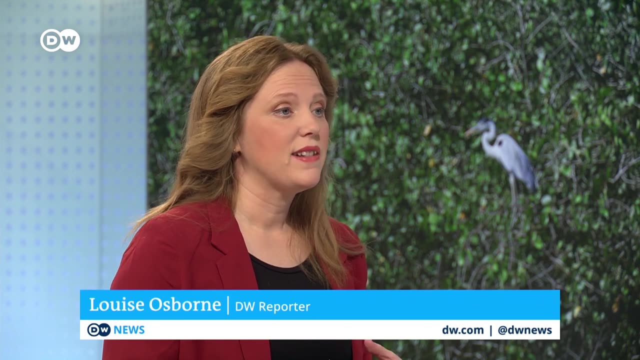 but surely there's more to it than that. Why else does biodiversity matter for health? Well, I mean, it's not just about, you know, dealing with when we're sick. Actually, it's much more essential in keeping us healthy in the first place. 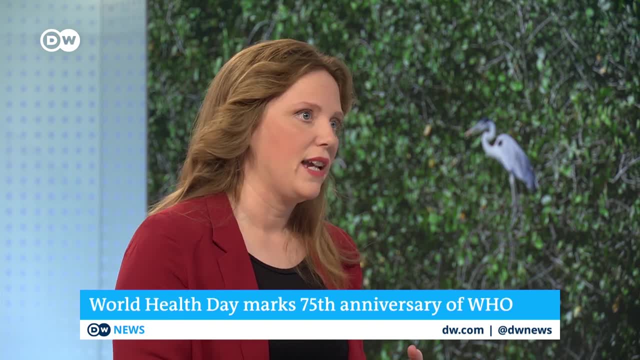 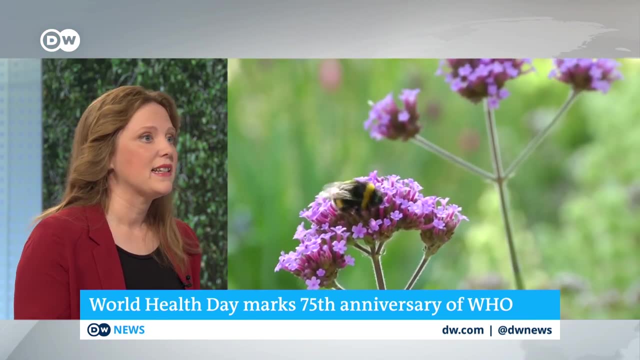 I mean, if we look at trees, for example, they take pollutants out of the air. There are studies that have shown in areas where there are more trees then air pollution is not such a big problem And obviously that is a big killer for humans. 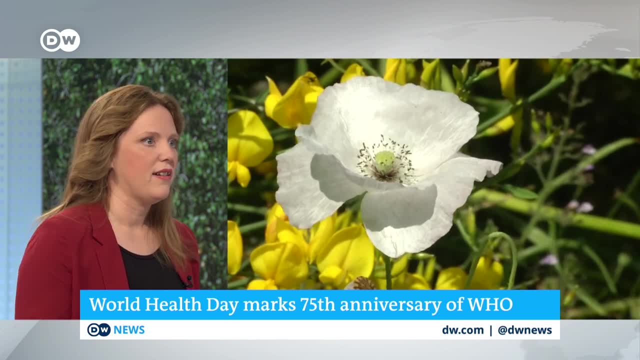 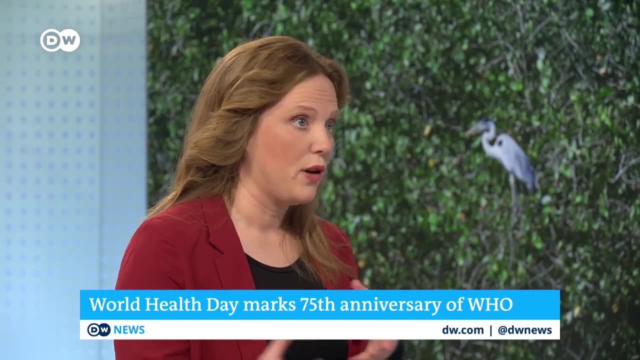 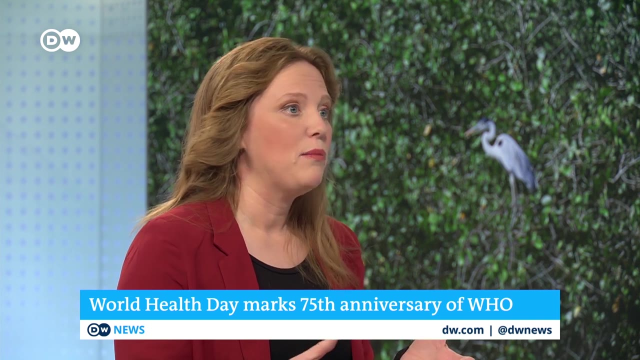 There's also wetlands, for example, that clean water. A city in India, Calcutta, uses wetlands to clean its water for farming and for other uses- for drinking. And again, clean water is a huge thing for human health, very important. 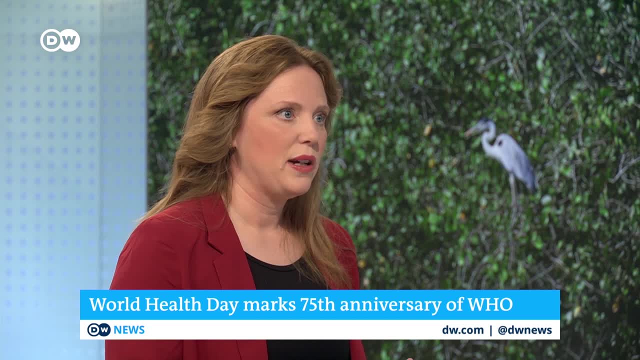 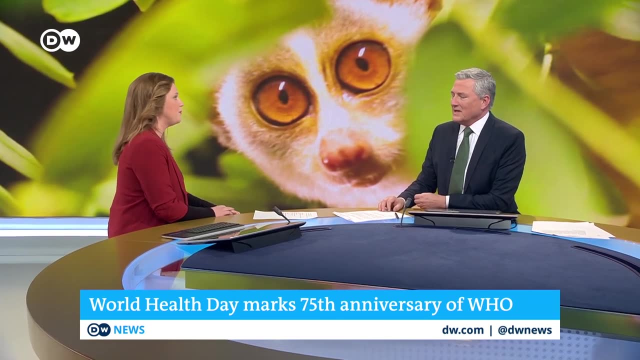 So there are all of these things, all of these jobs that nature are doing for us that you know we don't really even you know follow. And these are just a couple of examples. It seems intuitive, But we really should remind people. you know that. you know we don't really even you know follow. 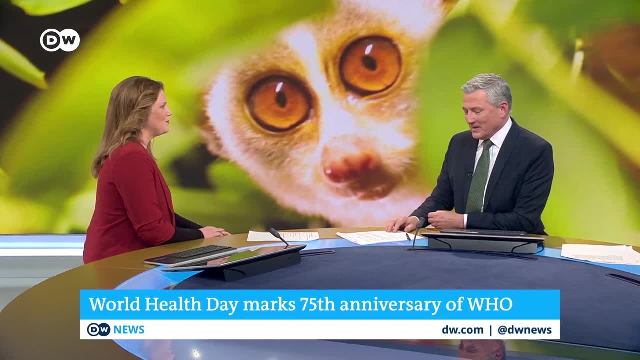 It seems intuitive, But we really should remind people. you know that, you know we don't really even you know follow, And we should remind ourselves from time to time to be conscious of it. Plants and animals, though, are disappearing. 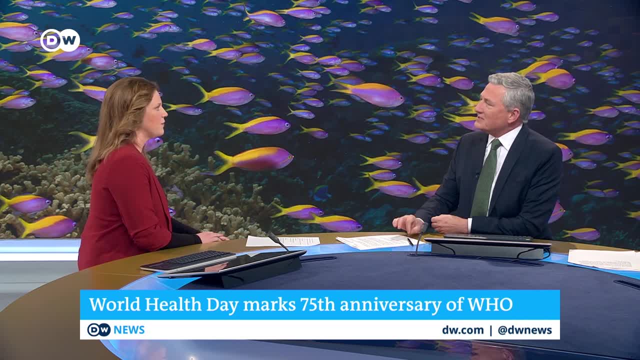 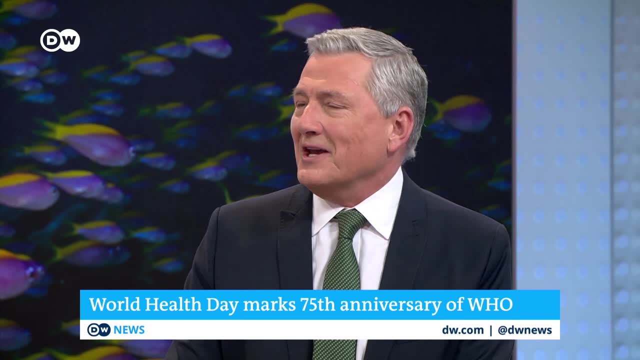 The species are disappearing at an alarming rate. At the same time, we're seeing technology advance by leaps and bounds, not least biotech. Can technology help make up for the loss in biodiversity? Well, you've probably heard about disappearing bees, for example. 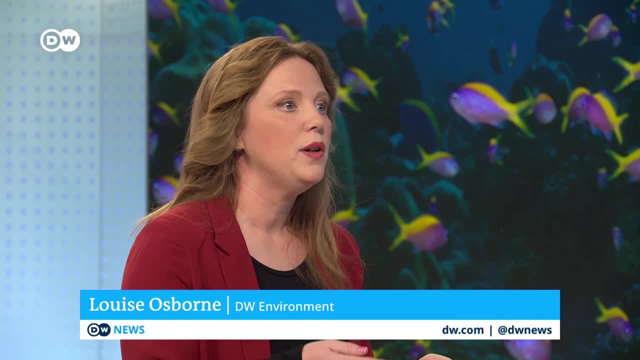 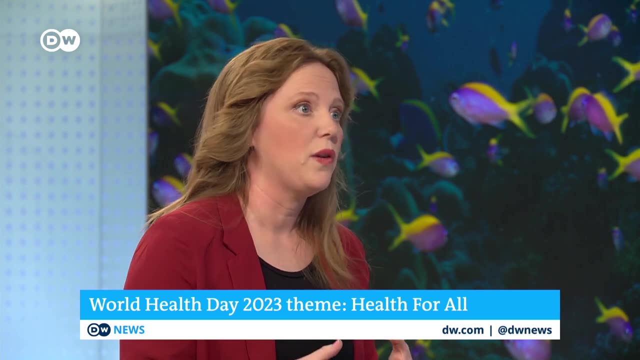 This is becoming an issue that insects are disappearing, and so we need those for our crops. There are machines that are being built, There are things that are being built that can pollinate our crops so that we're still getting food. So they're taking over the job from bees, for example. But I mean these are a lot more expensive And also they can't account for the complex interactions that animals have between each other and plants. So it's always difficult to say whether these things are going to be able to take over or not. 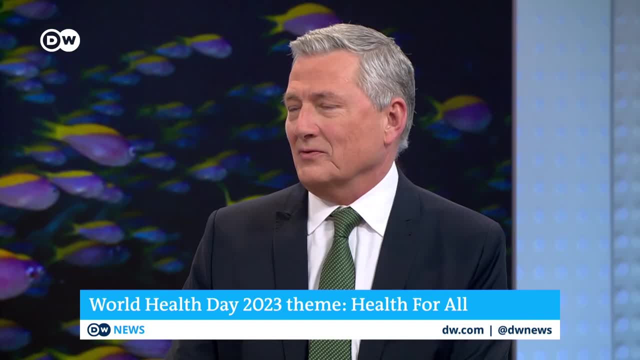 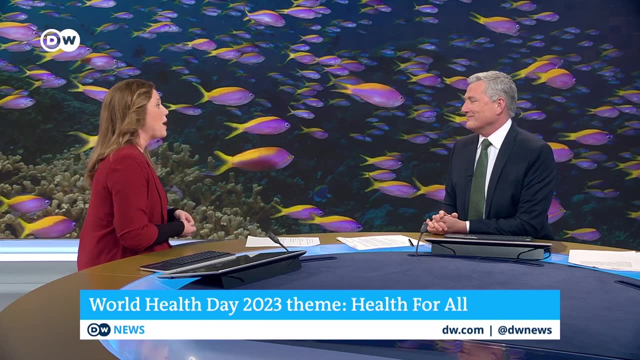 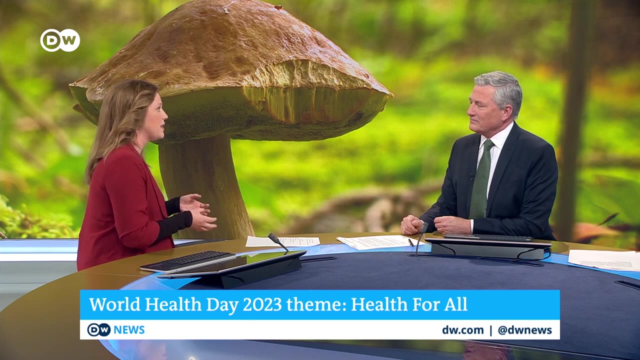 And what about efforts to keep nature intact, Louisa, To preserve biodiversity? Is there a reason to be hopeful? There are things that we can definitely do. Agroforestry, for example, is something where trees and shrubs and biodiversity are integrated into our farming practices. 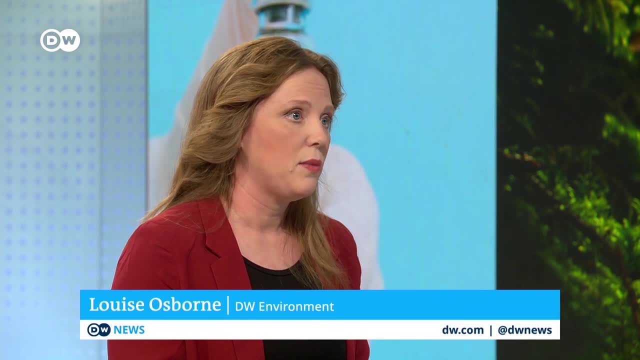 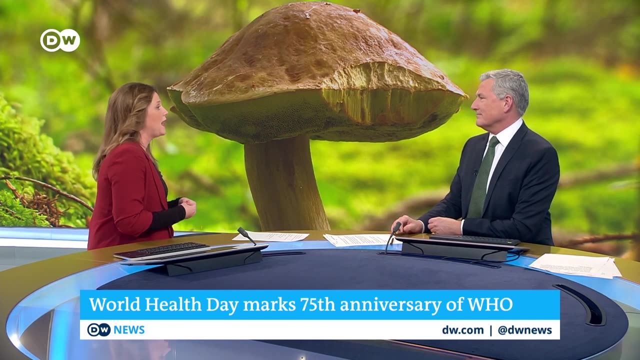 And obviously that is one of the biggest threats when it comes to biodiversity. As individuals, we can also look at our food waste, making sure that we are only buying what we actually need rather than throwing so much away. So there are all of these things. 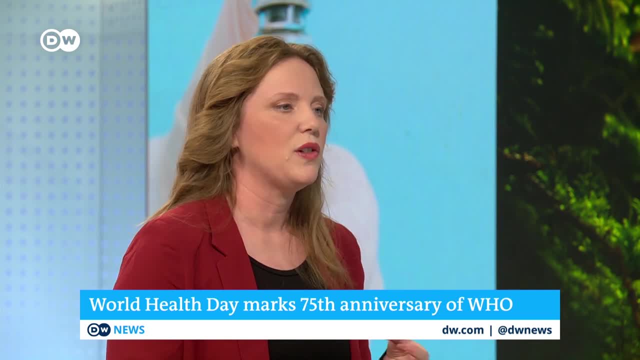 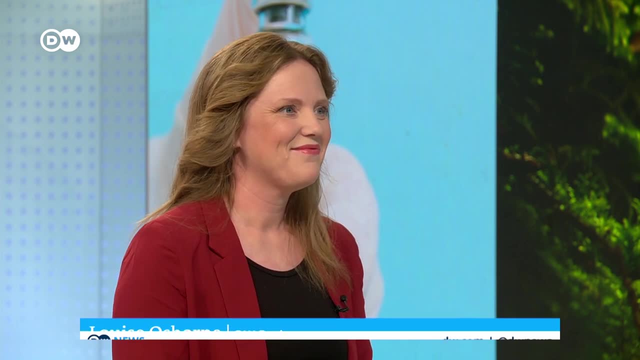 There are all of these things that can be done. There is no one solution, But combined together it will help. Louise Osborne from DW's Environment Desk. thank you so much.